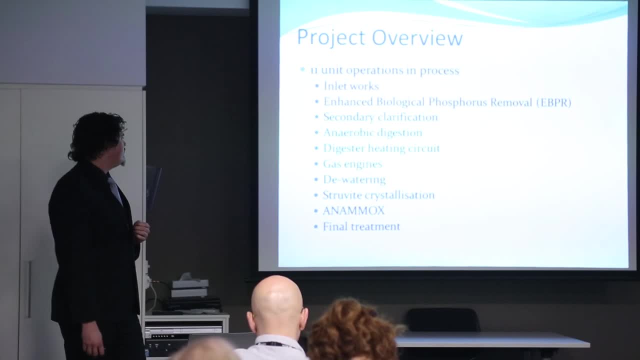 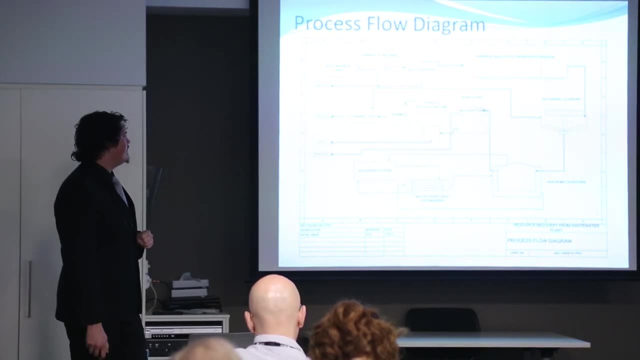 gas engines which run off the methane produced by the digesters, heating and watering, struvite crystallisation, an anammox process and then the final treatment stage. This is the PFD for our system, which I'll run through in a second with you. For our site. we have a few specific criteria which we were after in order to choose the correct location. The selection criteria for our site was a high predicted population growth of around 5% per annum, an ageing wastewater treatment facilities and an estimated population of about 300,000 by 2020.. 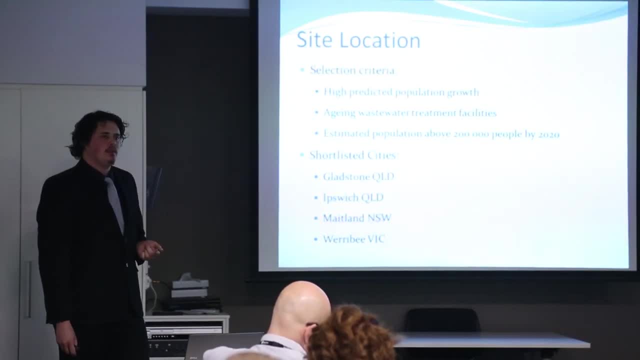 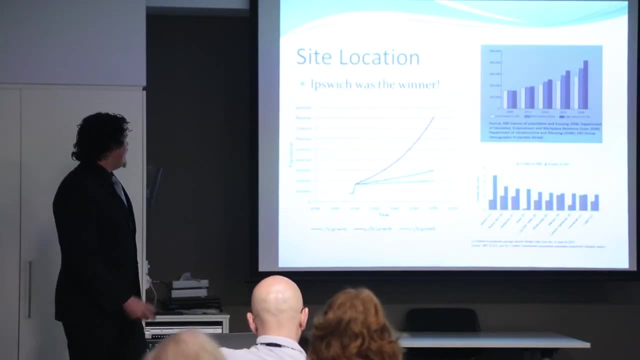 There were four shortlisted cities. that was, Gladstone in Queensland, Ipswich in Queensland, Maitland in New South Wales and Warington in Victoria. Ipswich was the chosen location. So here we've got three graphs. The first graph on the left hand side indicates our predicted population available or requiring wastewater treatment for our facility. As you can see, there is an initial spike, And that is assuming that one of the current older wastewater treatment plants, which currently treats 85,000 estimated population, will be closing down in 2020.. So that will be available for our system. 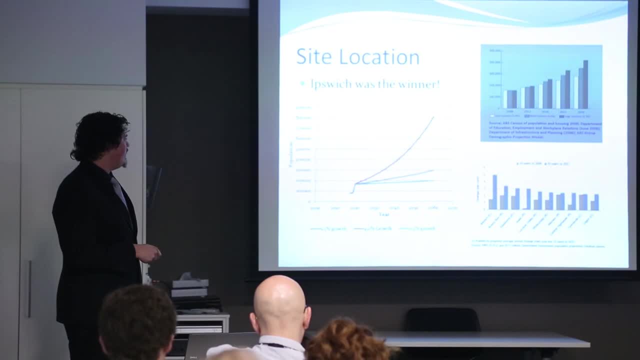 As you can see, we've done three different estimates of population increase: One at 4%, which is highly unfeasible, One at 1.5% and one at 0.5%. You should also know that between 2010 and 2017, when this starts- 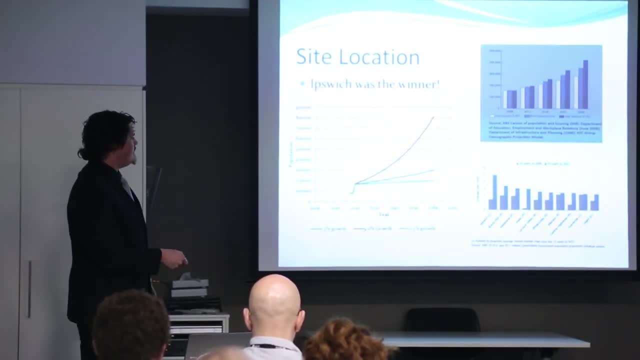 there is estimated to be a 4% population increase, Or up to 5% population increase. as you can see here, By 2020, the overall population in Ipswich should be over 300,000 people. This is the Ipswich Flood Control Council area. 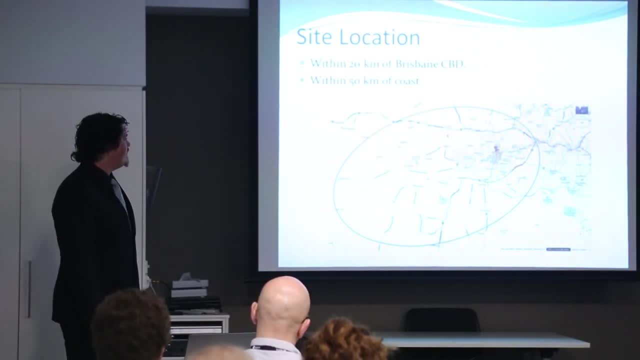 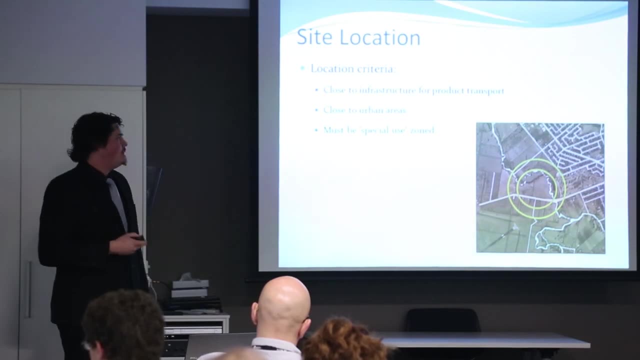 which is within 20 kilometres of Brisbane City and within 50 kilometres of the coast. The specific site we have chosen is right near the Amblin Military Base. So there's a few criteria before we just pick any site. It has to be close to the infrastructure of the product. 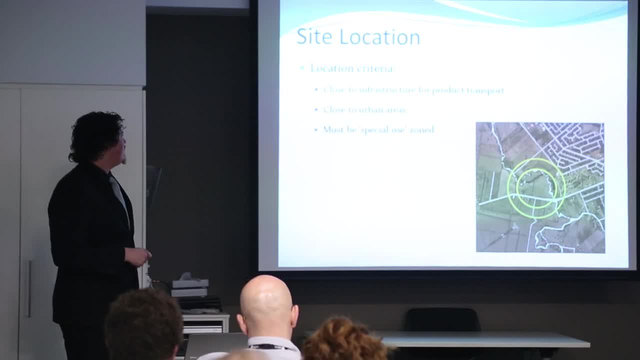 It has to be close to urban areas And it must also be, according to the council, zoned as special use. So, as you can see, this is the actual lot that we've chosen, And it has a 400 metre buffer zone between the actual site location. 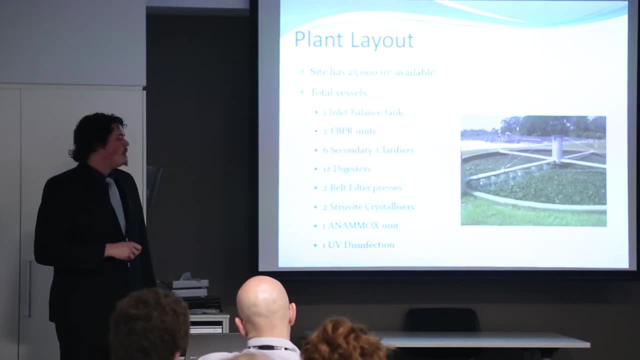 and the nearest urban population. For the site itself, it has 25,000 square metres available And, as you can see, we do actually have quite a lot of different vessels for our system. So I'll now run through the site layout for you. 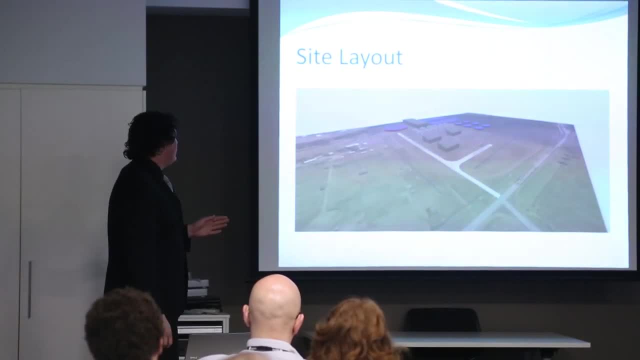 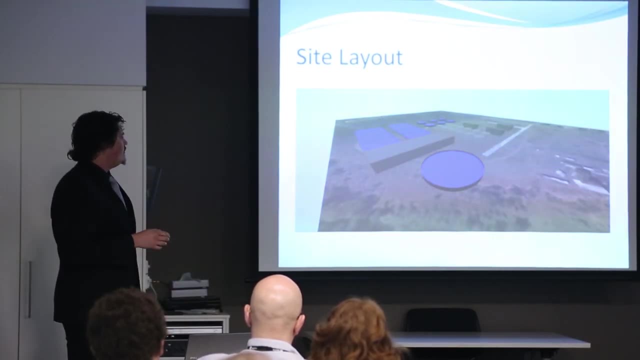 So, as you can see, our site will have a perimeter fence and an access road. Our first unit operation, or first section, would be the inlet fence, which is 100 megalitres. From there the flow runs into the inlet works. 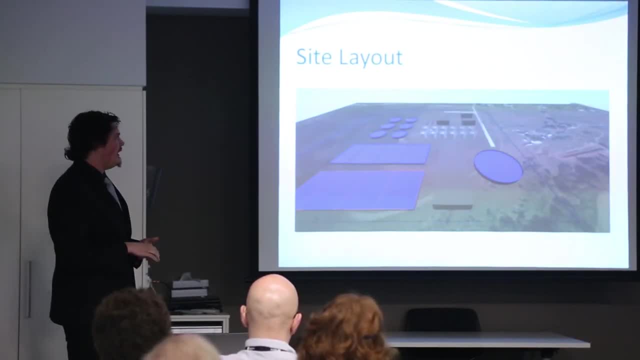 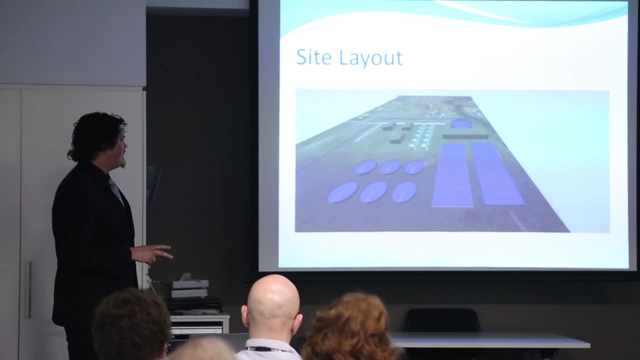 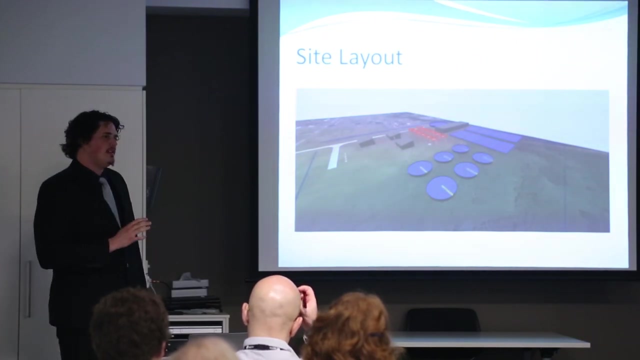 which comprises of adding a quick clarifier and primary separation. We then have our first unit, which is our enhanced biological phosphorus removal. This is split into two different sections to enhance our reliability. Then it runs into the secondary clarifiers, which is split into six different units. 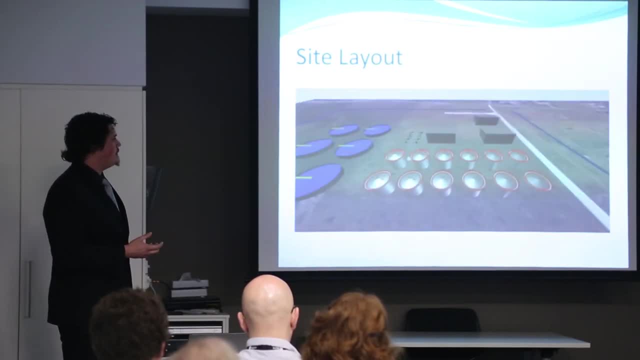 Again to enhance or to optimise the process. From there, the effluent runs into the anaerobic digesters which produce methane. The methane is then fed into the gas engines which they use to offset our internal power generation. The effluent from the digesters runs into the deep watering system. 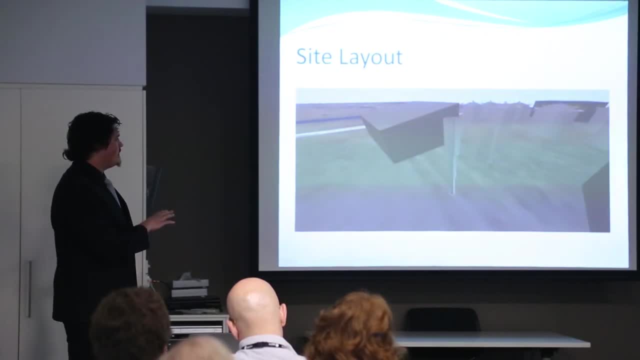 where the solids are then transported out and the effluent runs into our strubite crystallisers. After the strubite crystallisers, the effluent runs into our anaerobic system, which then goes into our final treatment. As you can see here, this is the location for our site offices. 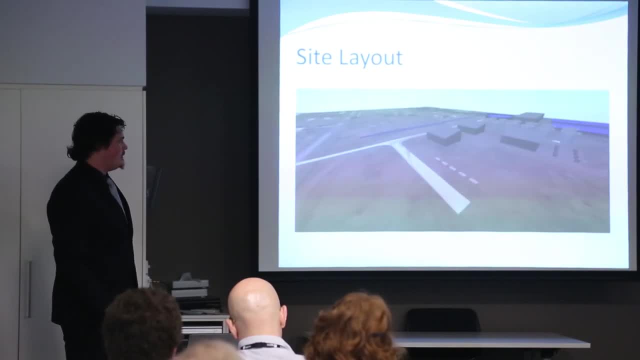 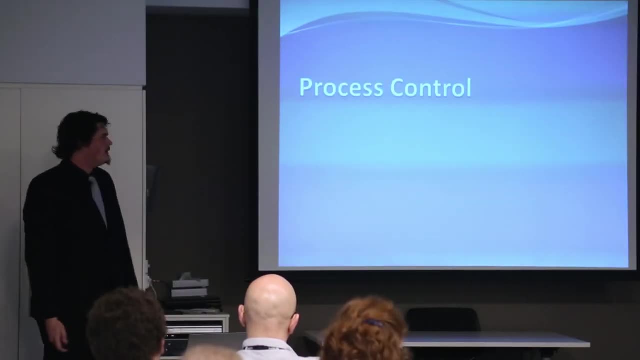 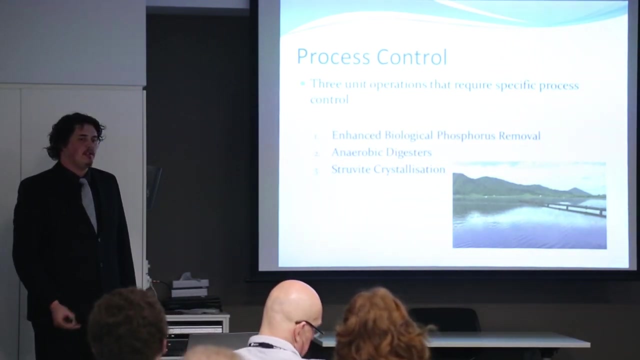 and this is to give you some scale. That is the size of a single-denominable office unit. I'll now run through the process control for our system as well. For our process, we have focused on three major unit operations which require specific process control. 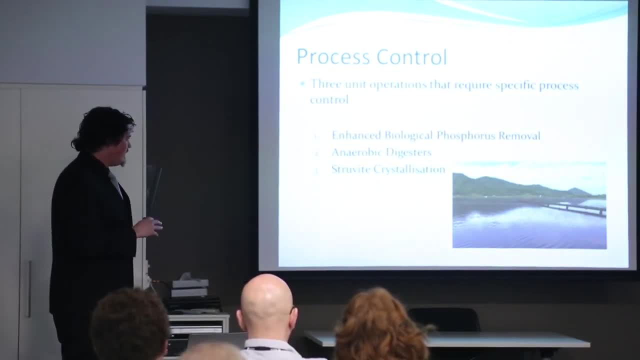 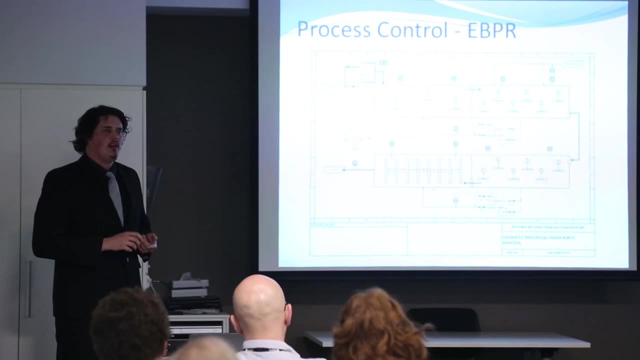 Most of the unit operations do actually require process control, but these are the three we've had specific focus on. For the enhanced biological phosphorus removal, a few of the main characteristics that need to be observed are the residence time within the system, as well as the dissolved oxygen within each of the units. 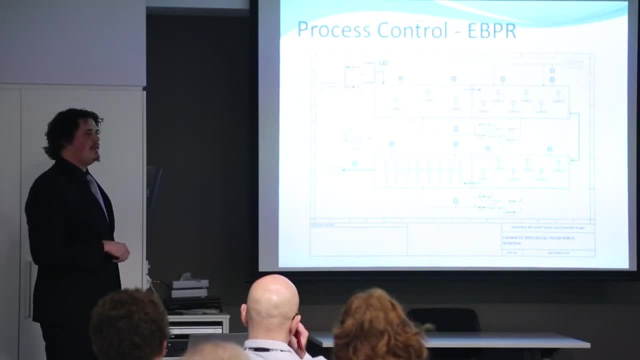 As you can see, we've got a feedback loop between our inlet pumps and the flow transmitter, which monitors the inlet flow rate. The effluent then runs through all four stages of the system, with a loopback between stage two and stage one. 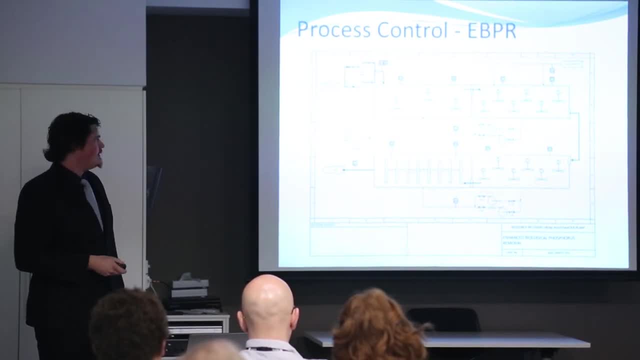 again feedback controlled by the flow transmitters and then a loopback between stage four and stage three. Within stage four it is actually an aerated system, so it does actually have dissolved oxygen sensors which run back to the blowers, which allow for monitoring of the aeration within that system. 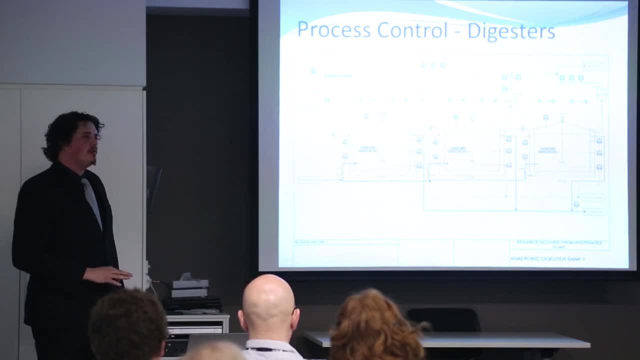 For the anaerobic digesters, there are quite a few parameters you need to control. A few of the specific ones are the temperature within the system. So there is actually three specific temperature probes at different levels within the digester itself, which then feed back into a feedback loop. 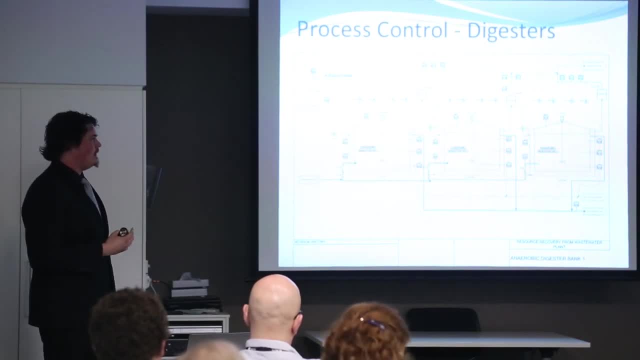 which runs off the anaerobic digester, water jack heating system, So that will allow for a temperature control over that. We also have a nitrogen purge for the anaerobic digesters. This allows for, say, start-up and shut-down. 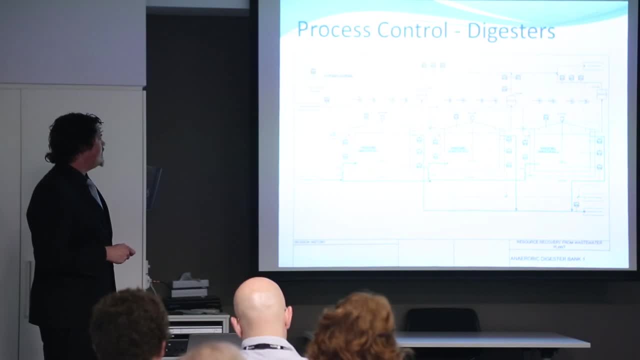 methane being a fungible gas, And then we also have monitoring on the outlet composition of the gas as well. With these two biocrystallisers, two of the main parameters you want to look at, or look at control within the system. 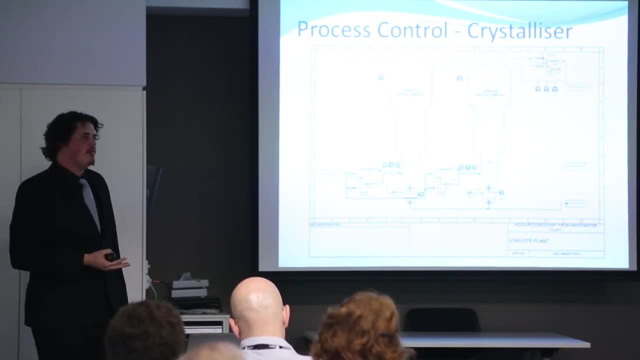 are the inlet flow velocity, so the minimum fluidisation velocity of the system, as well as the pH. So at the inlet there's flow streams again which do run back to the pumps to keep it at a constant speed, And then the inlet will also be kept at. 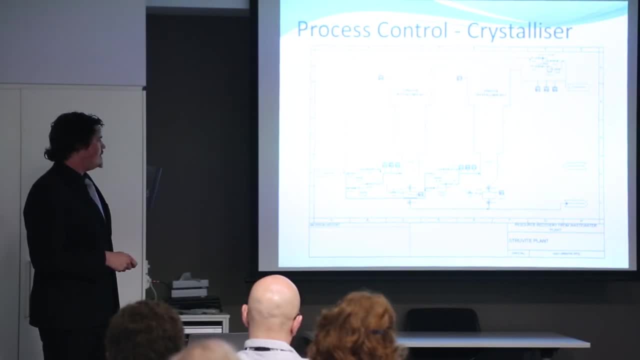 sorry. the inlet pH will also be monitored with a feedback to the pH level Which goes into the system. At the outlet for the crystallisers there is a feedback loop which goes around back to the entrance of the crystallisers which allows for nucleation of the true biocrystals. 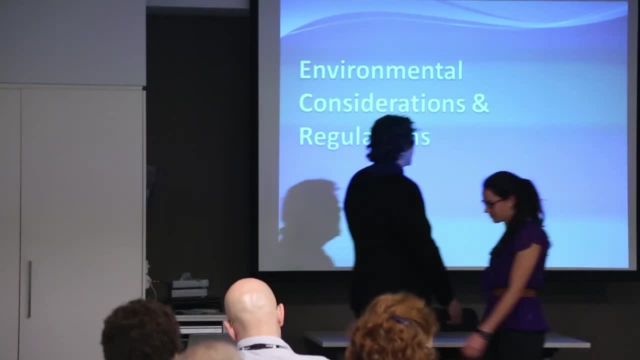 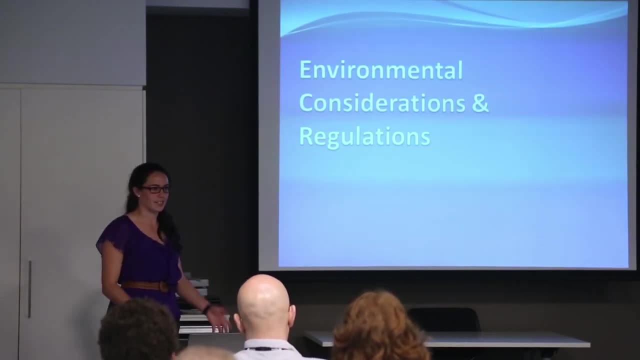 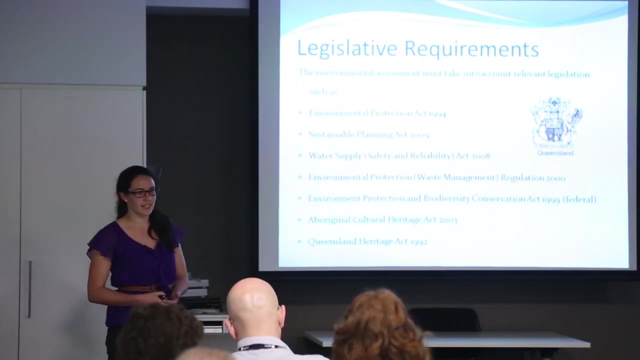 May I pass that over? I've been looking at the environmental considerations legislation and regulations that we need to follow for our solar treatment plants. We've looked at over 25 pieces of legislation and I've just listed the main ones that are important for this sort of plan. 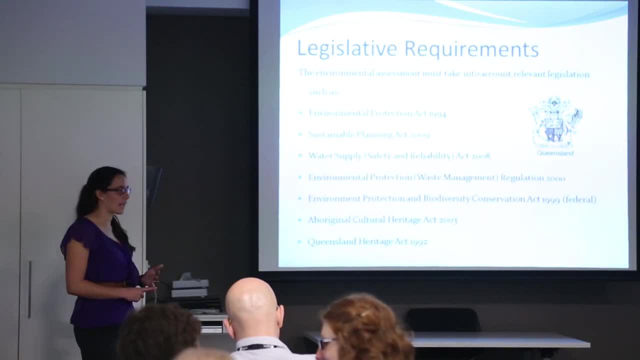 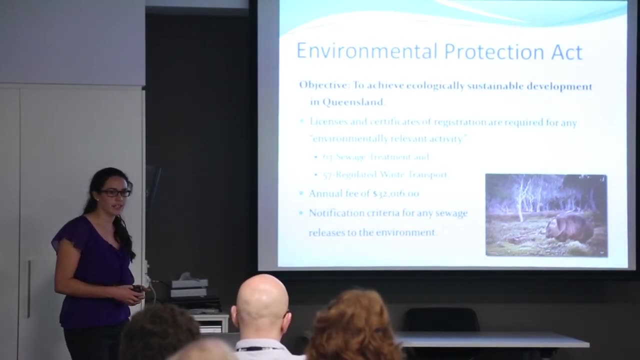 This is specifically the Environmental Protection Act, the Sustainable Planning Act and the Water Supply Act. Some more detail on the Environmental Protection Act: The objective is to achieve ecologically sustainable development in Queensland. The Act: our licences will be under this Act. 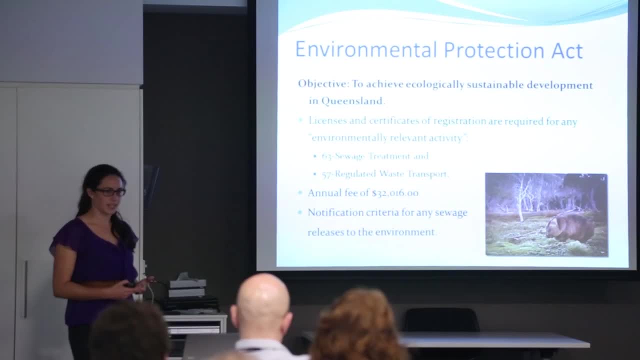 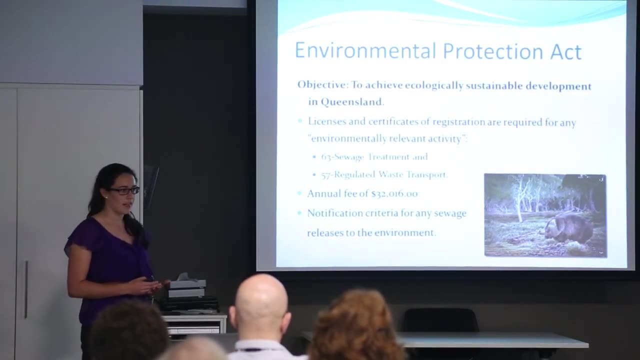 We need a licence for the sewage treatment and also for the regulated waste transport, which will be the biosolids. It says our area fee, which will be $32,000 for a plan of this size, and also specifies environmental release certification to the relevant authority. 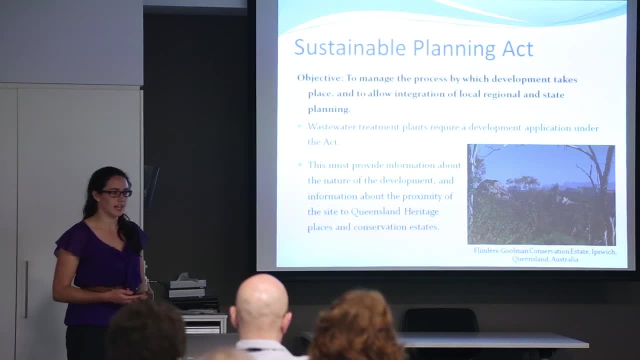 The Sustainable Planning Act is the Act we'll have to submit our development application under. This takes into account conservation estates in the area as well as heritage sites, And we've checked this out. There are no conservation estates within the specific site area. we're looking. 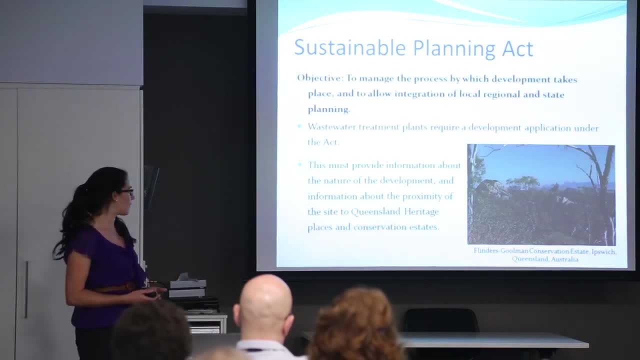 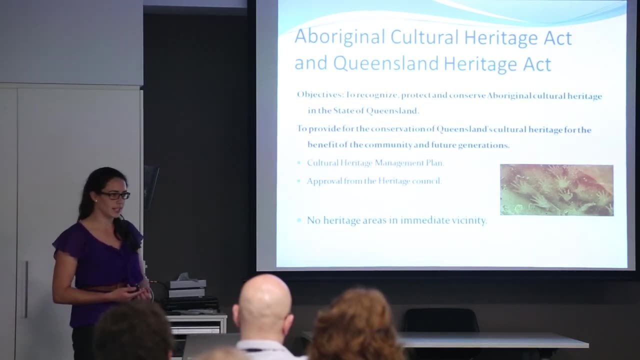 There's also no native carbon plants and no flora or fauna under threat. We've also had a look at the Aboriginal Cultural Heritage Act as well as the Queensland Heritage Act. It's important to make sure there are no heritage sites where we're building. 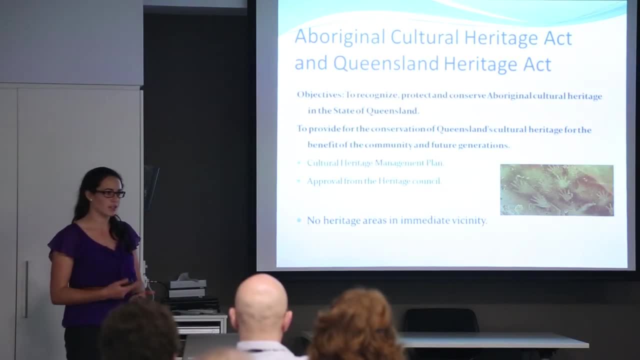 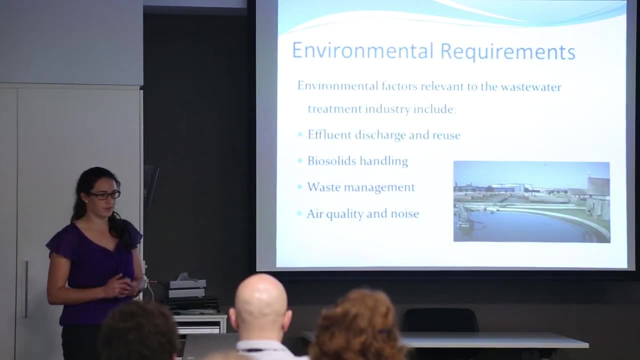 If there were, we'd need approval from councils and to create some management plans, But as it is again, we've selected a site with none of these issues. The environmental requirements for a wastewater treatment plant are quite important there: The effluent discharge and readings requirements. 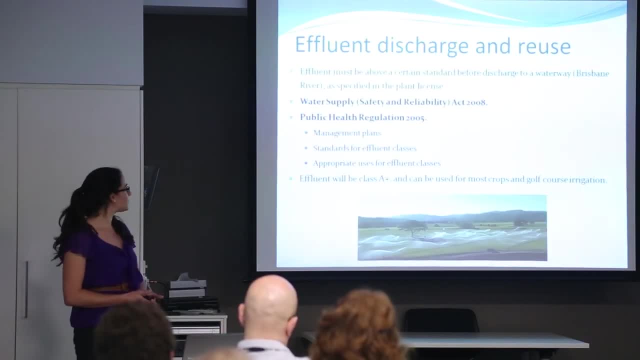 excellence handling, waste management and air quality and noise. So for effluent discharge and readings, this is regulated by the Water Supply Act and the Public Health Regulation. Obviously, the effluent that's discharged to the river has to be of a certain standard. 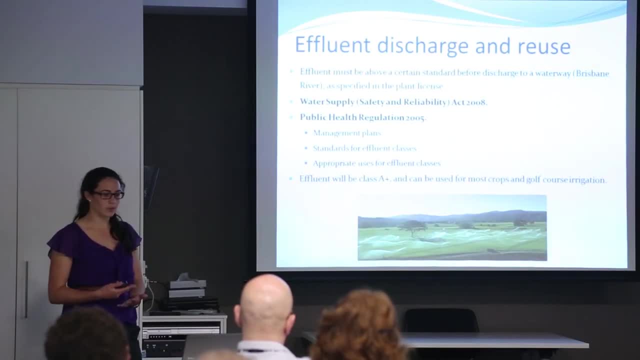 We'll have a licence which will specify the criteria that we have to meet For the readings. this comes under the Public Health Regulation. There's specified management plans required and it also sets out the standards for the various classes of effluent, And our design plan will be achieving an A-plus class. 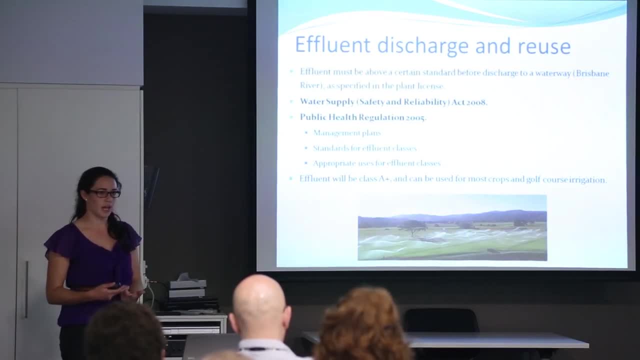 This means that if we're using it for agricultural reuse, we could use it for irrigation for most types of crops, as well as Gulf Coast irrigation or irrigation at the air base nearby. It gives us a fairly wide range of reuse options With our biosolids. 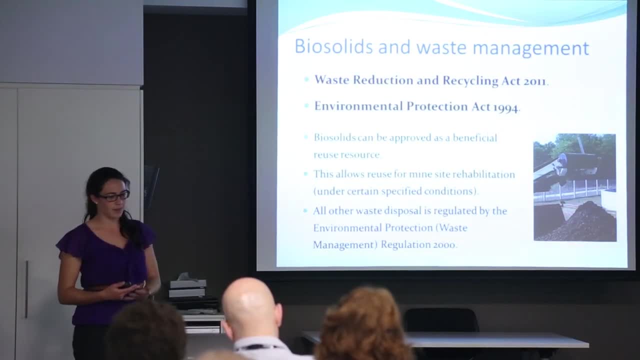 the Waste Reduction and Recycling Act, as well as the Environmental Protection Act, regulate the biosolids reuse. Currently, Queensland has a new management plan where they encourage the qualification of biosolids as a beneficial reuse resource. This allows it to be approved under certain conditions. 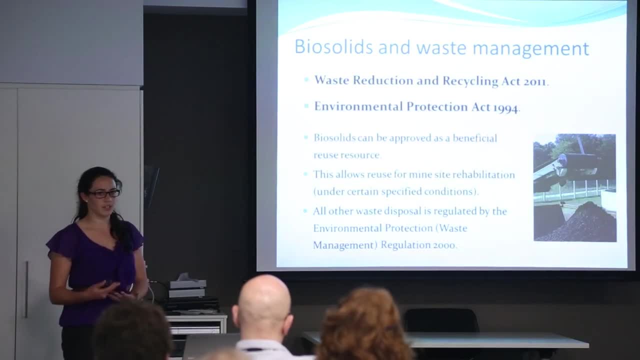 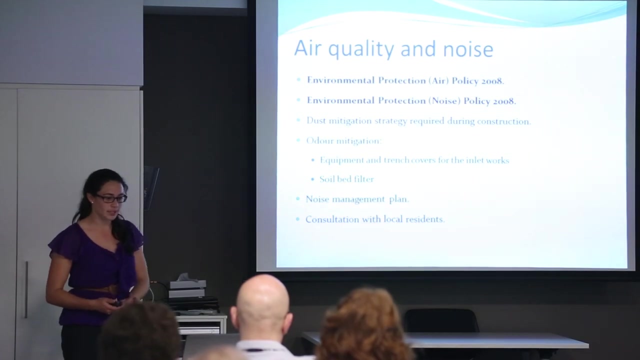 as a resource rather than a waste product, and it means we can use it for mine site rehabilitation. All the other waste disposal from screenings or grid classification is regulated by the Environmental Protection Regulation. Air quality and noise is regulated by Environmental Protection Policies for air and noise. During construction, we'll require a dust mitigation strategy and odour considerations always coming to play with a wastewater treatment plant. Firstly, we'll be covering equipment and trenches in our inlet works, which is where most of the odours are generated. If this is insufficient, 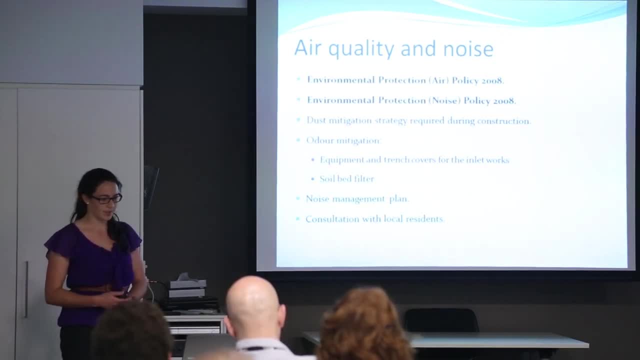 we'll be able to install soil and vegetable seeds as well. We'll have a noise management plan specifically for construction, as we are in the area of residential homes, and then we'll stay in constant consultation with the residents to ensure they know what we're up to. 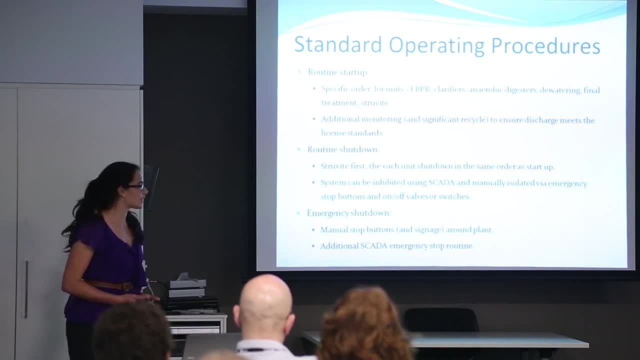 Have a look at the operating procedures. For the start-up. a specific order is required. Firstly, to see the EBPR system, which is our secondary treatment with biomass from another plant, and just fill this section until it is running and actually treating our waste. 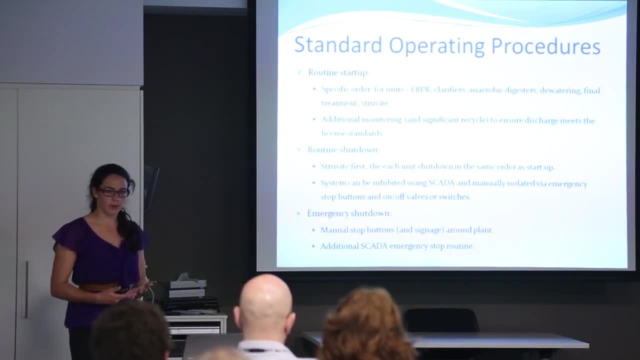 Then we're able to start up the clarifiers, the anaerobic digesters, our dewatering process and our final treatment process. And the street art will be the last to come online During the first few months of operation. additional monitoring: 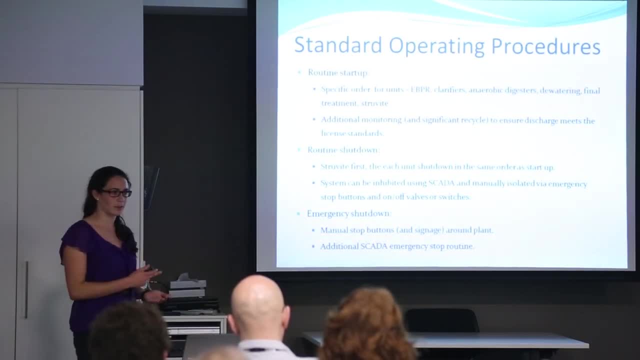 and probably quite a large amount of additional recycle through the plant will be required to achieve the effluent standards specified in our licence For the shutdown. the street art system will be shut down first, and then each unit will be shut down in the same order. 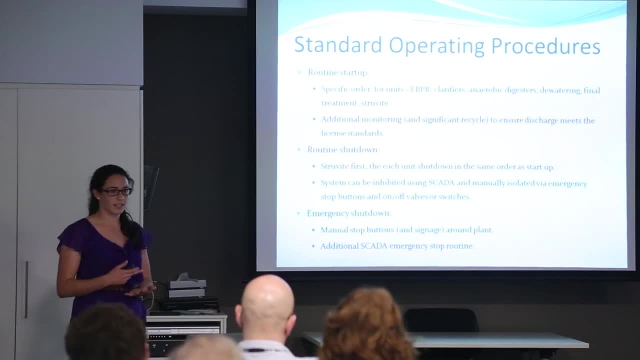 as they were started up. This shutdown can be done via our SCED system. There'll also be manual on-off switches and buttons around the plant For an emergency shutdown. we'll obviously have emergency stop buttons at every unit operation and signage And we'll also have a standard emergency stop routine. 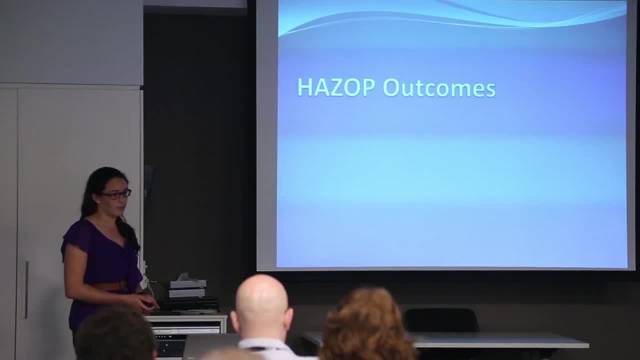 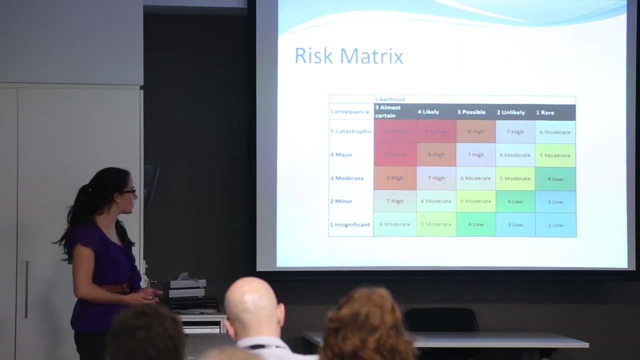 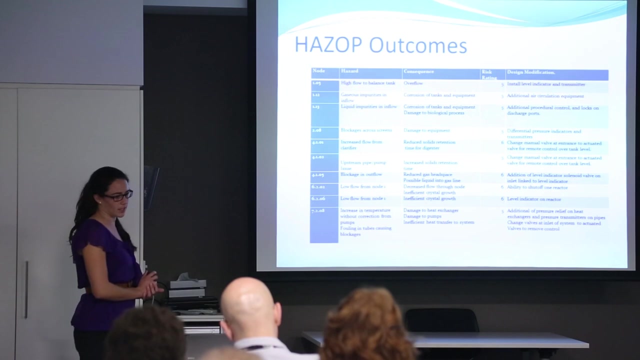 set into place. So we've performed a hazard to investigate the risk and safety of the plants with our plants. This is the risk ranking matrix that we've used. We decided a risk above a five or a moderate requires extra mitigation strategies. So here is an example. 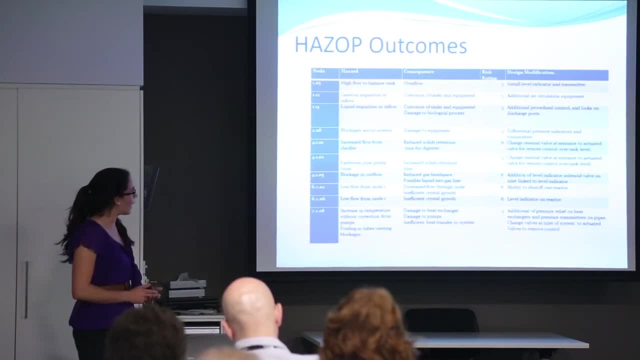 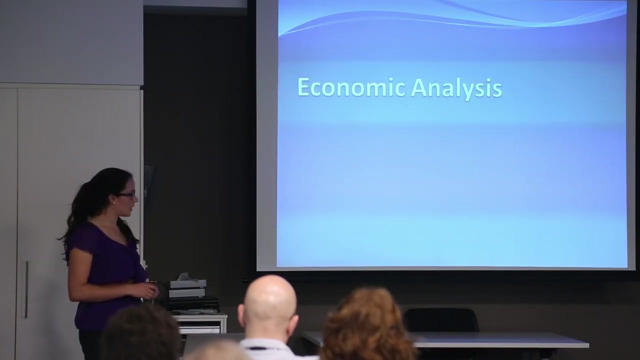 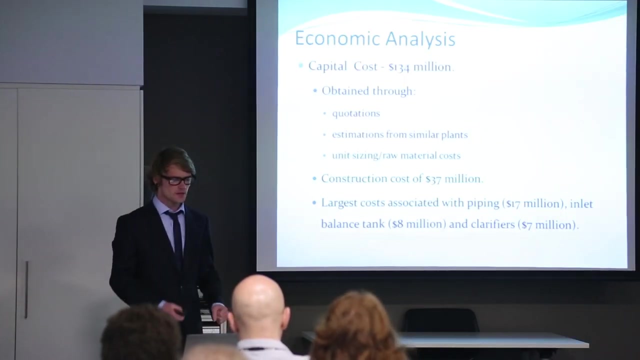 of some of the risks that we've identified and our risk design modifications range from just installing loading the containers and transmitters through to installing extra equipment or procedural controls that need to be enacted. I'll pass on to Alec for the economic analysis. I'll give an overview of our economic analysis of the plant. We split our economic analysis into three major parts: The capital cost of the plant, the operating cost and the income generated by the plant. The total capital cost was $134 million. This was obtained through quotations from companies, estimates from similar plants and unit sizing and raw material costs. 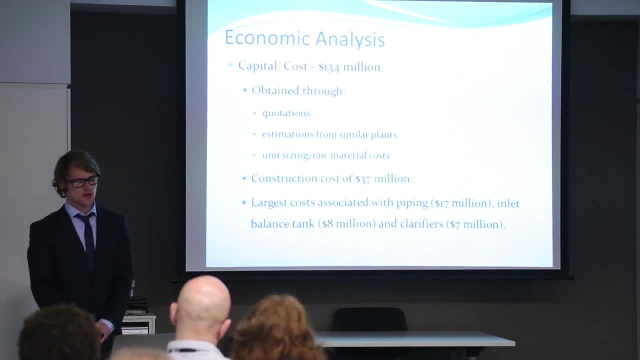 from phase two design paper. The construction cost of the unit operations themselves was approximated at $37 million, And these largest costs were associated with the piping, which was $17 million, the inlet balancer, which was $8 million, and the clarifiers, which was $7 million. 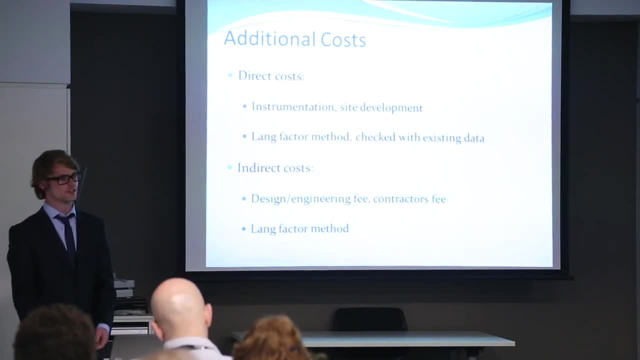 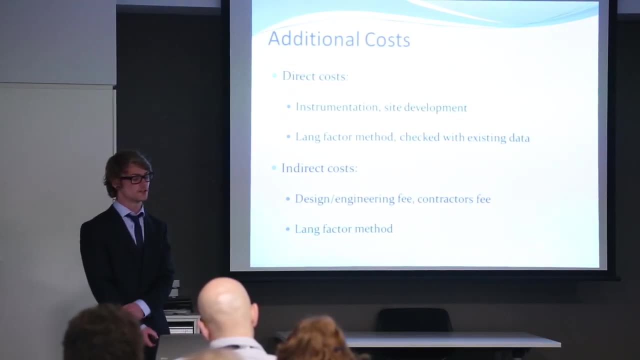 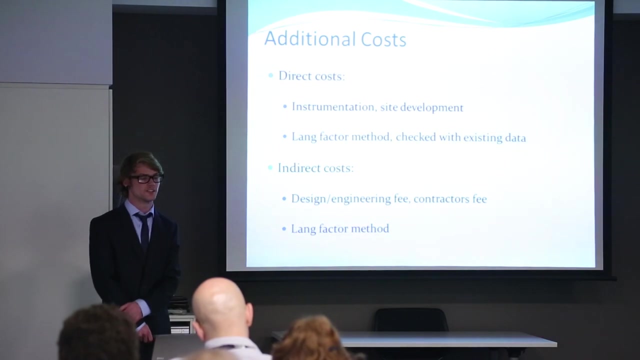 This construction cost was also included additional costs of direct and indirect nature. The direct costs included things factors such as instrumentation and site development, And these were calculated by the lane factor method and checked with existing data where possible. The indirect costs were the design and engineering fees. 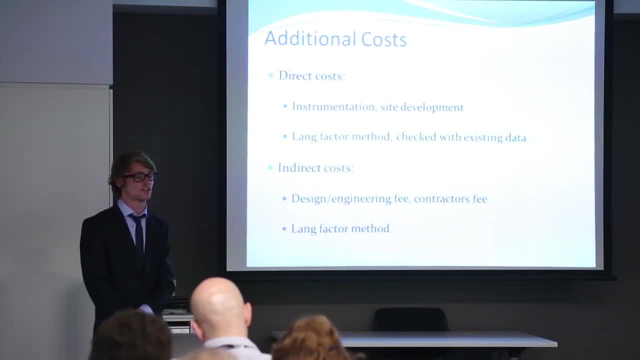 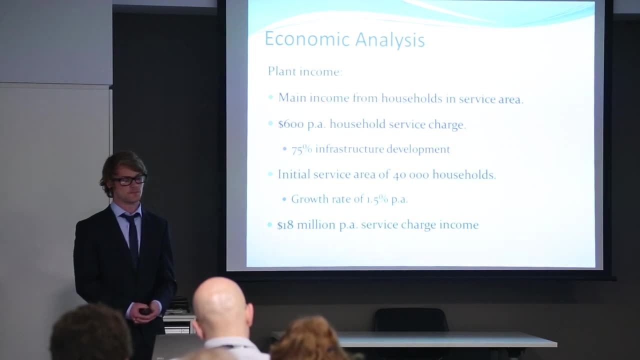 and, excuse me, the contracting fees. And this was also calculated by the lane factor method. The plant income: The plant income was from the households in the service area of the plant. This was from a water bill. We obtained a $600 per annum household service charge. 75% of this was going to our plant, so $450 per annum per household. In the initial service was 40,000 households And so this related to an $18 million per annum service charge coming to us, And then obviously that would grow. 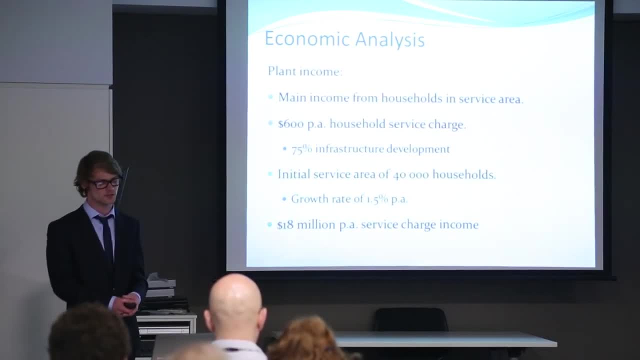 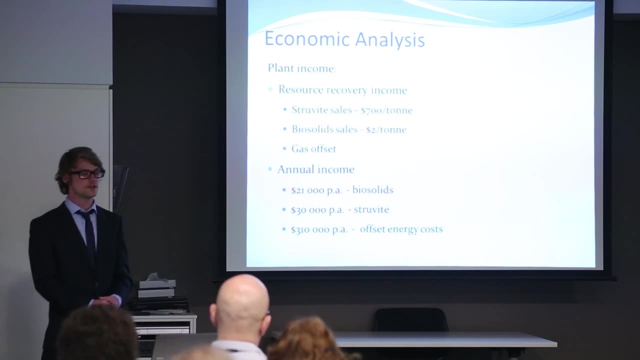 to our growth rate of 1.5% per annum households, It starts to take into effect. We also got income from our resource recovery. Struvite sales were taken at $700 a tonne. Biosolid sales were $2 a tonne. 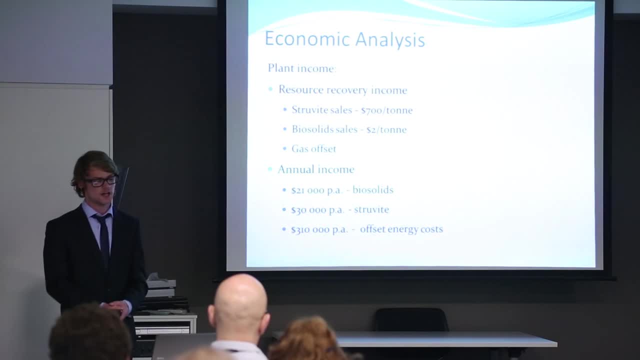 And we also obtained offsets from our gas engines. This related to an annual income from $21,000 for biosolids, $30,000 for struvite and $310,000 offset energy costs, And obviously this is per year. Sorry, offset energy costs. Now for the operational costs. The operational costs were calculated to be $4.3 million per annum. This is split up into maintenance costs, which is $1.8 million per annum. Operating labour, which was $680,000 a year. Chemical addition which consists of the flocculant for dewatering, sodium hydroxide and magnesium chloride for struvite. That was calculated at $100,000. And the power for the plant was calculated at $1.5 million a year. 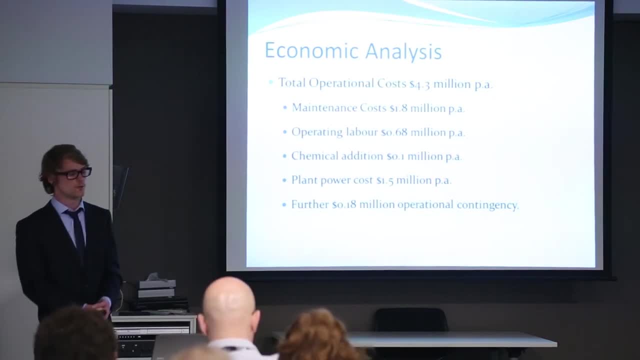 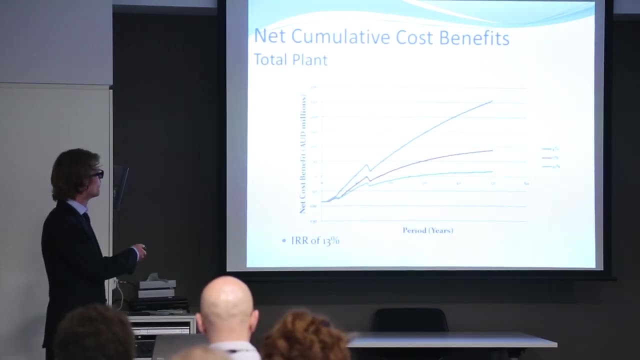 We also allowed a further $180,000 for operational contingency. We also did a net present value analysis, as you can see in this graph, for 4%, 7% and 10% discount rates. You see the internal rate of return. 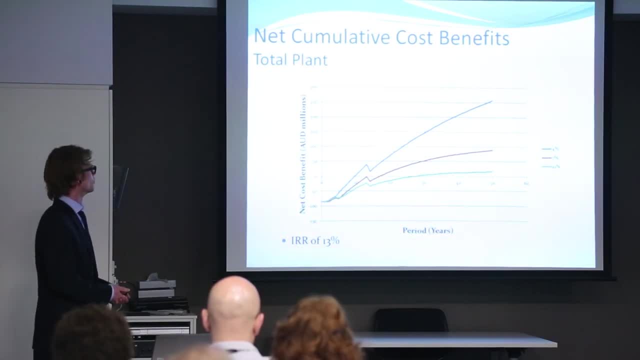 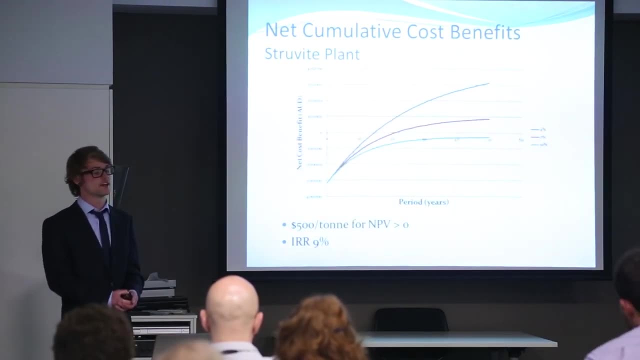 was calculated to be approximately 13% And all reasonable rates, the plant was able to pay itself off. We also did a net present value analysis for the struvite part of the plant in particular, because we wanted the struvite to be stand-alone and pay itself off. 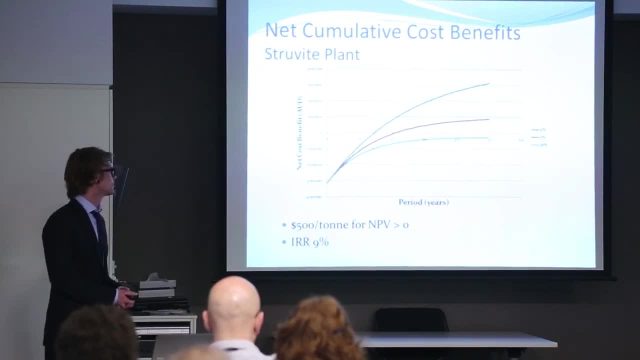 As you can see here, this is for a $700 a tonne price. We also did 4%, 7% and 10% discount rates. You'll see the internal rate of return is 9% on the struvite. 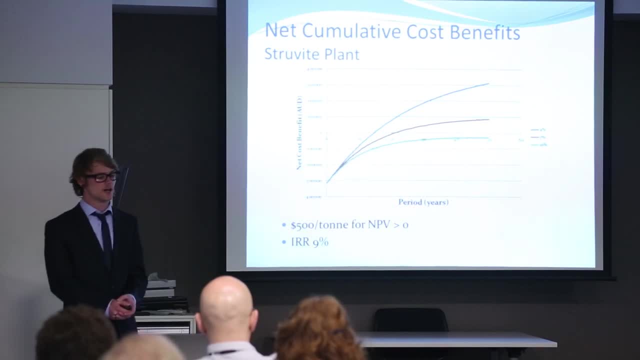 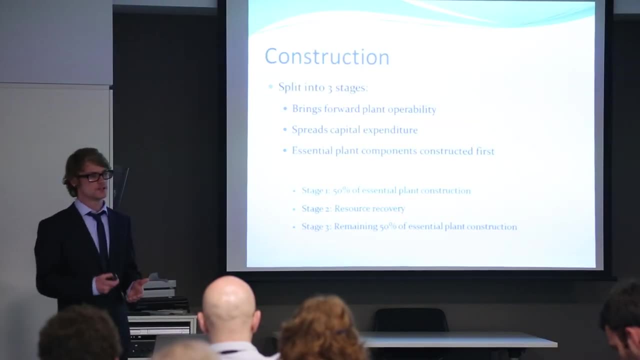 And we also discovered that under $500 a tonne the struvite will not be able to pay itself off. Now we go through the construction schedule. We split the construction in three stages. This brings forward the plant operability. It spreads the capital expenditure over many years. 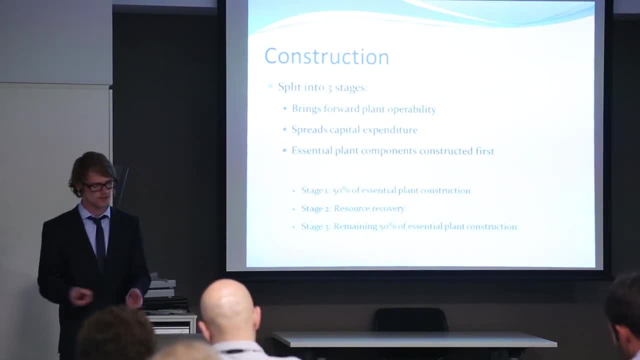 and it allows the essential plant components to be constructed first, then the resource recovery. Stage 1 consists of 50% of the essential plant construction. Then stage 2 will consist of the resource recovery sector And then, in stage 3, the remaining 50%. 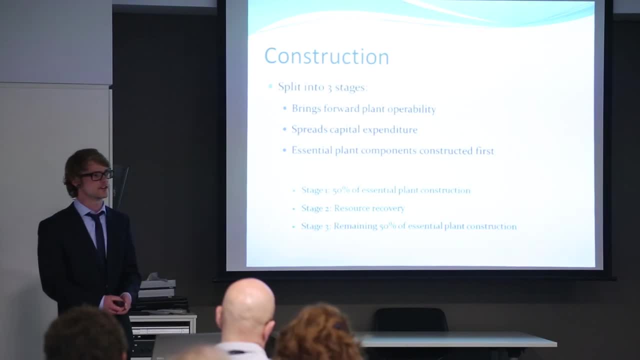 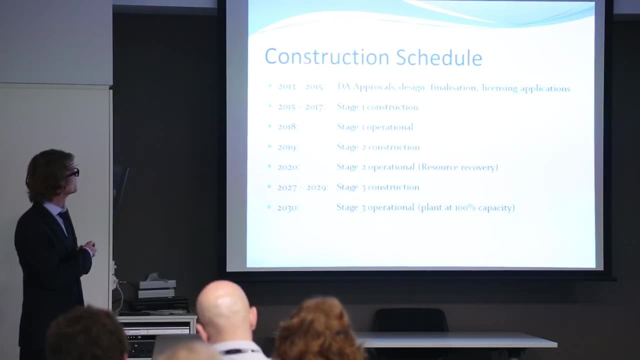 of the essential plant construction will be completed, hence leaving 100% capacity of the plant being operational. Here's a timeline that we can see: The DA of Crickle's design, finalisation and licensing applications will be commencing from 2013 to 2015,. where stage 1 will begin construction in 2015,. take approximately two years, so 2017.. Once that is completed, in 2018, it will be operational. Then stage 2 will be construction in 2019, taking one year to complete. 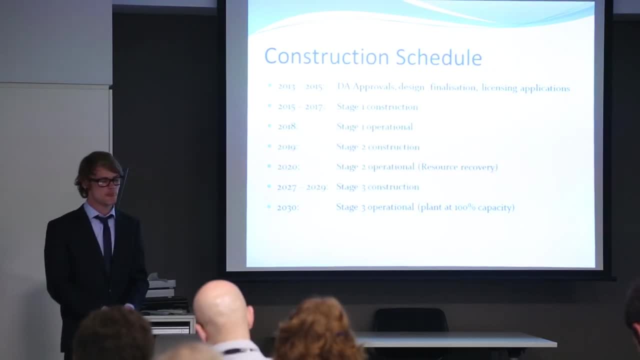 which will then be operational in 2020.. Then stage 3 will be completed in 2029, taking two years, and then it will be operational in 2030, which leaves the plant at 100% capacity. Just for a quick conclusion. 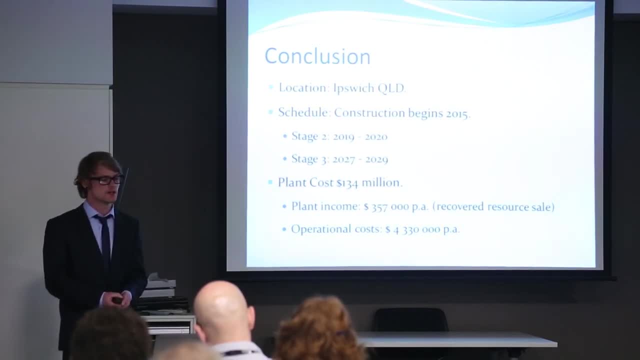 we chose this switch Queensland as our site location. The construction begins for the plant in 2015,, with stage 2 beginning in 2019, ending in 2020, and stage 3 beginning in 2027, ending in 2029,. where full-scale operation of the plant will be able to be resumed there. The total plant construction cost is $134 million, with plant income from resource recovery $357,000 per annum, and the operation cost associated with the plant is $4.3 million per annum. 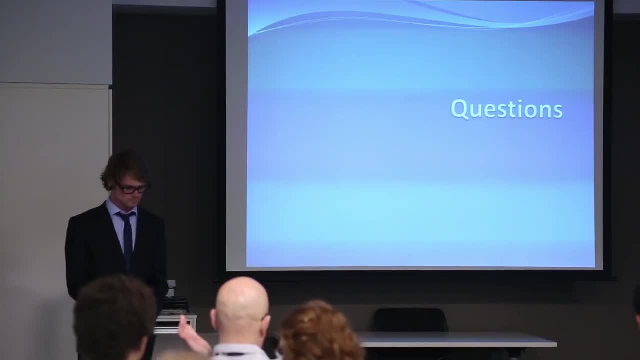 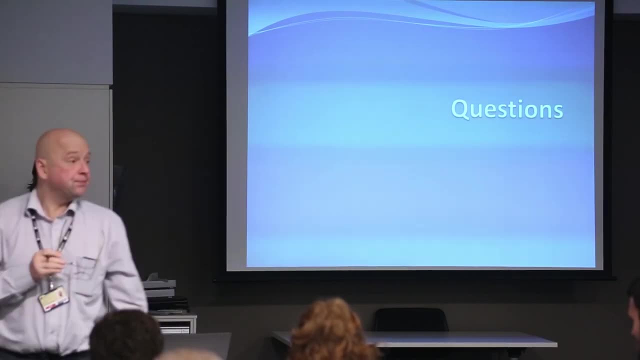 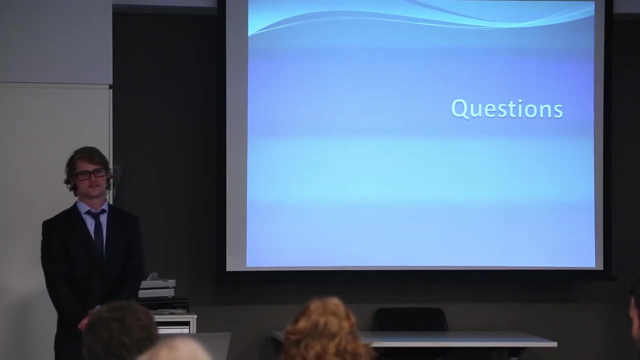 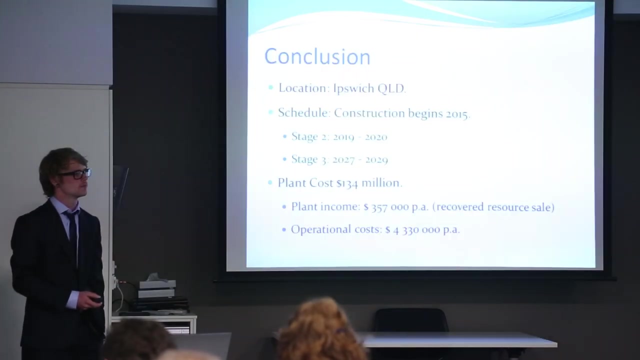 Thank you, Thank you. Thank you very much. Any other questions Go ahead. What is Drupal? Magnetic phosphate fertilizer would go into the slow-release fertilizer. Geoffrey, You know, on the first line you had something about high-flow steam balance. 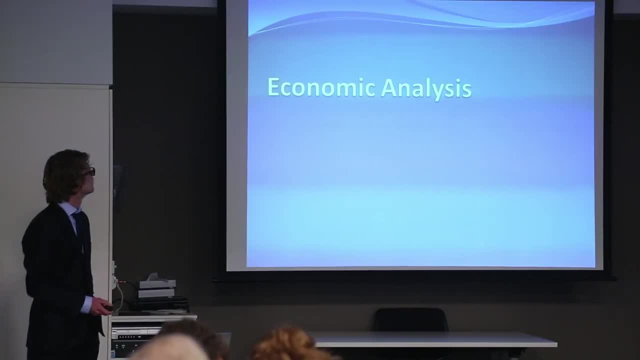 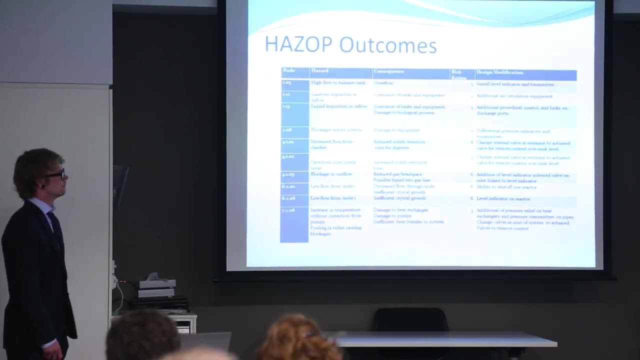 This is just a quick example of some of the hazards that come across. So what happens in a wet-weathering event where you get stream flows coming into the plant? So during a wet-weathering event, there's actually a bypass system which will allow. 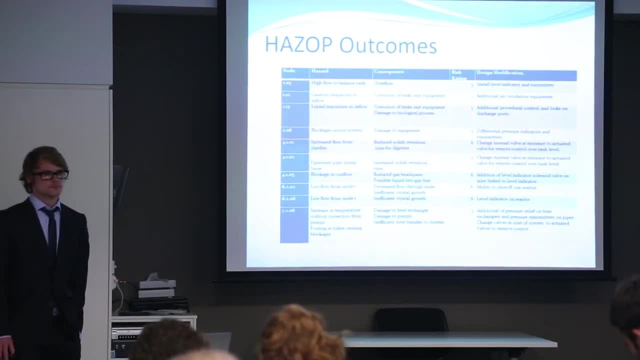 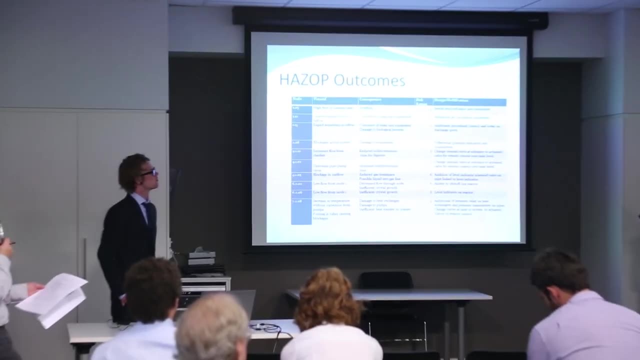 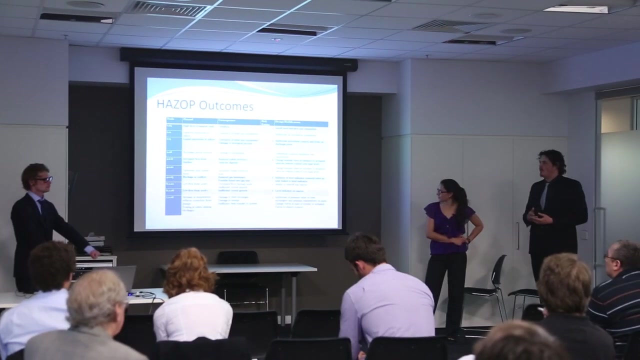 just after the primary separation, which will bypass directly into our final effluent. Due to the treatment standard, which is A-plus for the effluent, we'll actually be able to water that down and reduce the quality of our effluent just during peaks of increased flow into the plant. 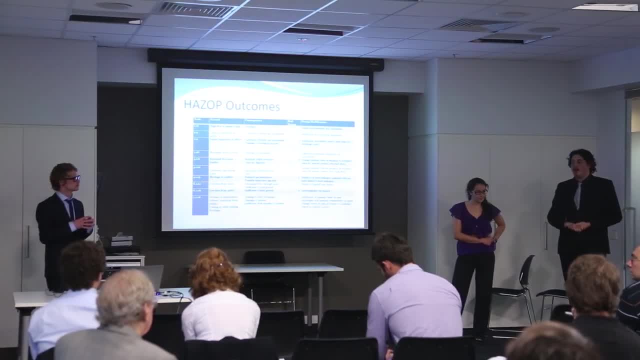 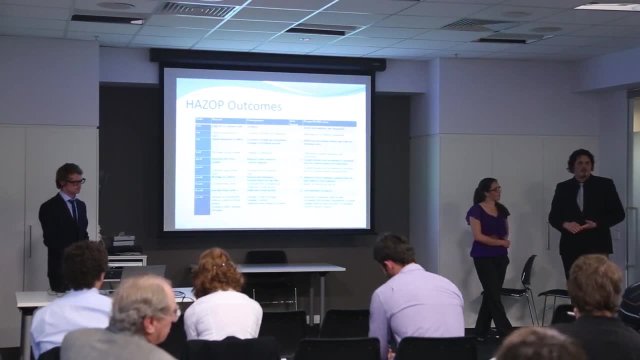 Okay. So when does that water then go to In our final years? Well, the water comes in. we're discharging the water and we've got a recycled water stream where, hopefully, some of it will go to farms and stuff like that. 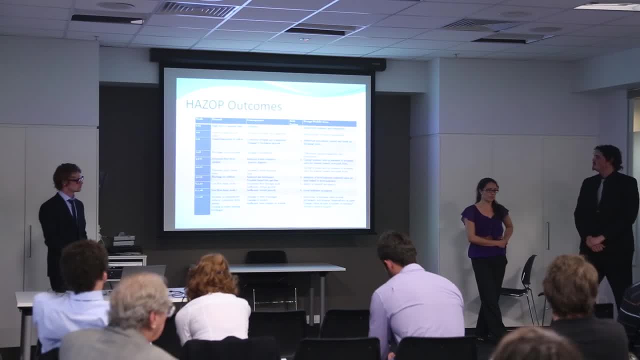 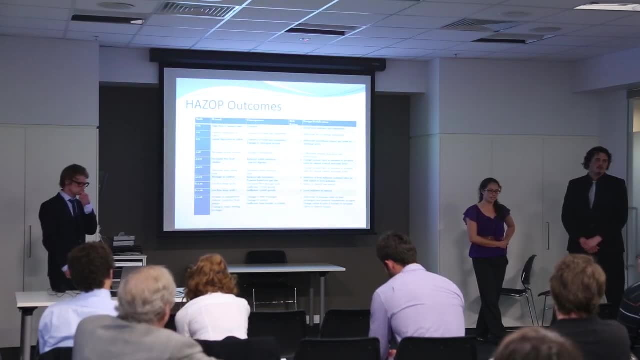 Yep, We can also have. we've got space on our site for ponds to create high-holding ponds in the case of high-flow events like extreme flow events. But unless it is extreme, hopefully, I think our balance tank has been sized quite. 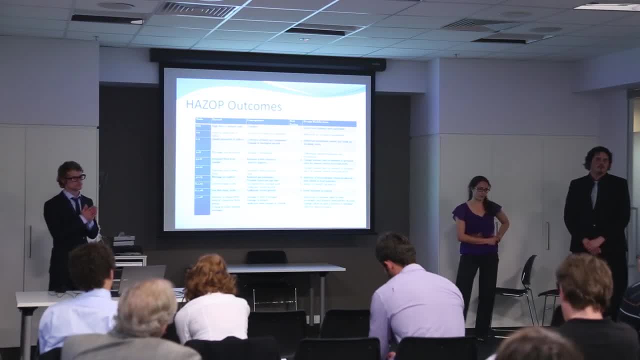 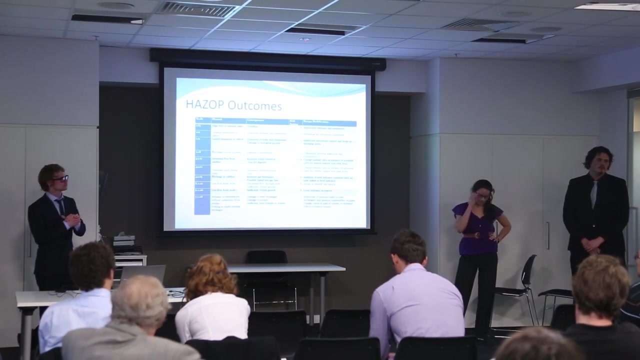 quite considerably large to hold the most high flows. Okay, So the balance tank wouldn't operate at its full capacity. It has the ability to store 100 millilitres, which is like a full day's worth of flow. So could. but what happened to the balance tank used for? 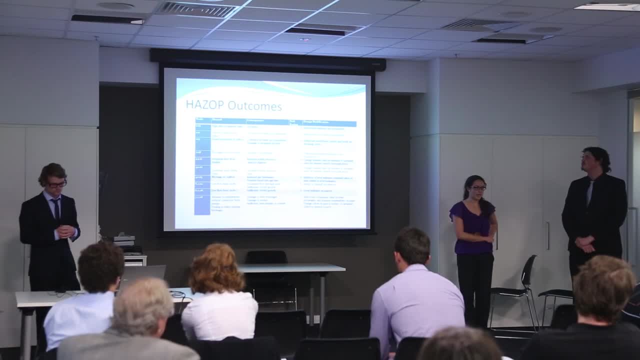 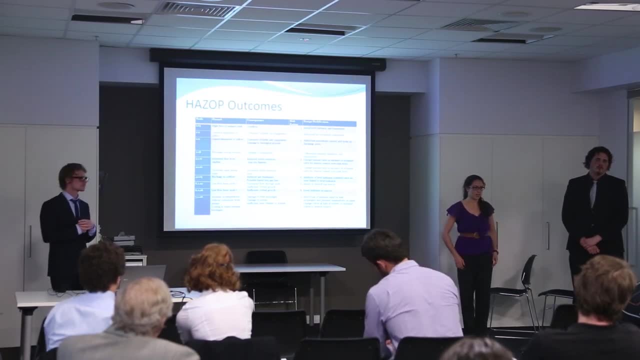 We haven't used it on site storage ponds And if, Which is beyond the scope of this, Yeah, we haven't designed those, But there is room on the site to construct storage ponds now which we'll be able to hold for these high flows. 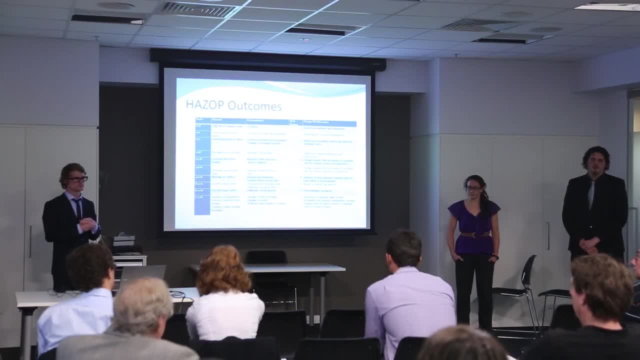 Go on. I guess a question in a similar vein: What happens if the gas turbines go offline? Is it going to have an impact on anything? Yep, So it's highly unlikely that all the gas turbines will go offline, So that's why we've actually chosen eight. 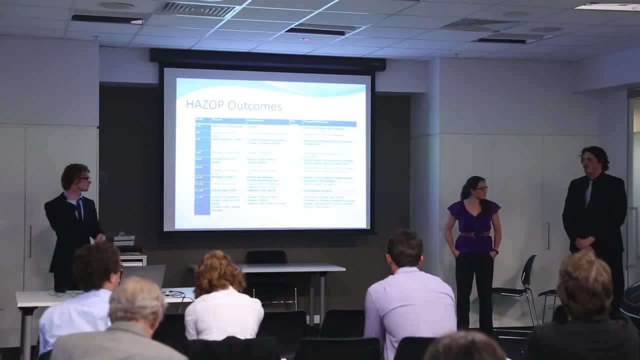 in that they are actually oversized, So not all eight will be running once. It's only going to require six, So you have two spare. The other thing is there is methane storage there, So that's why we've actually chosen eight, in that they are actually oversized. So not all eight will be running once. It's only going to require six, So you have two spare. The other thing is there is methane storage tank on site as well, So I think we've got multiple layers of redundancy in there. 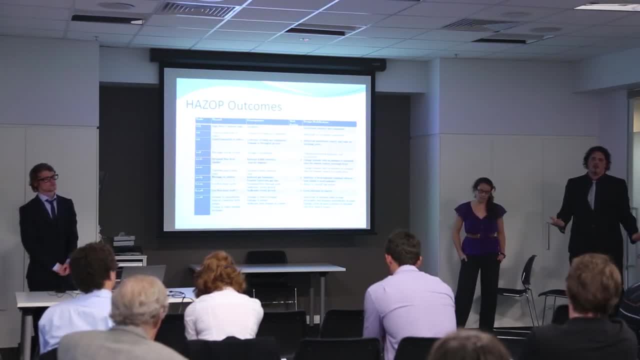 How do you store the methane on the high pressure? We didn't look into that in this design, And this is going to be turbines- or is it gas engines, Gas engines? So we looked into both and we decided on gas engines, I guess. 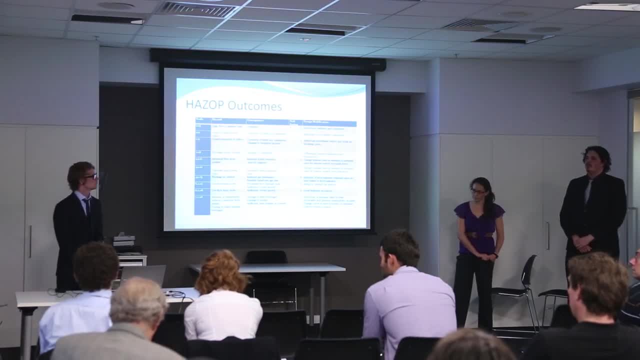 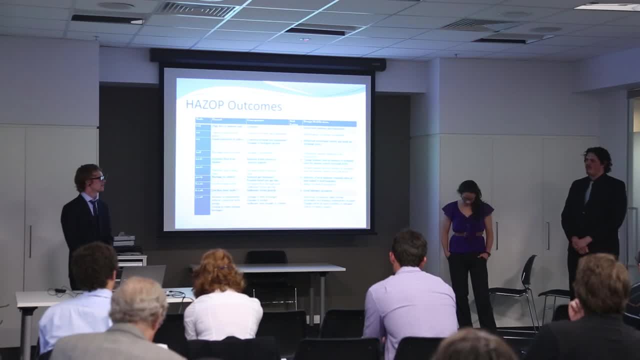 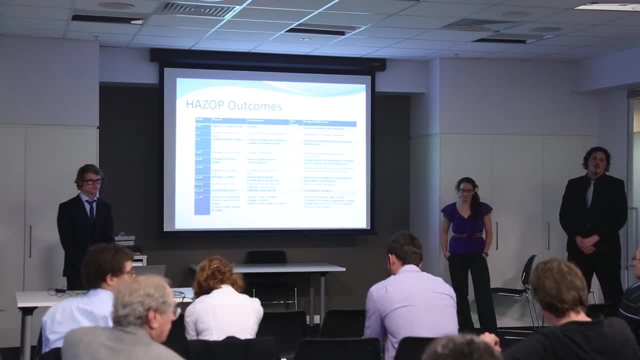 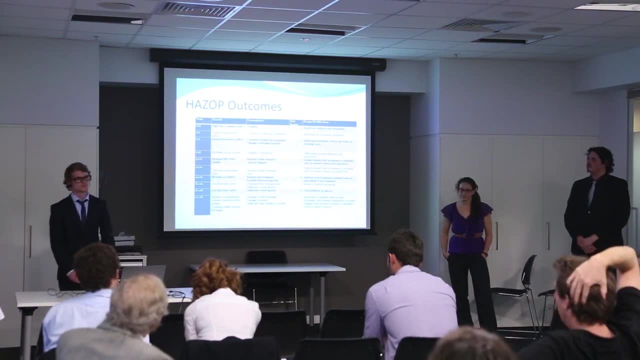 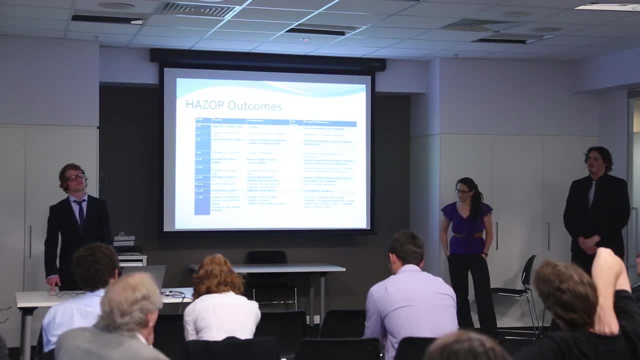 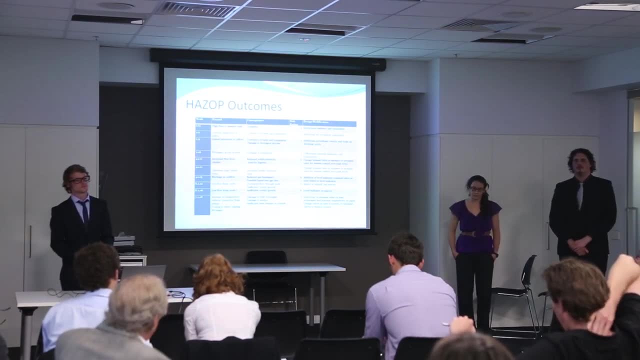 I think it was about $6,000. It ended up about $45,000 an hour per person. So if you've got $6,000 or $7,000 an hour, roughly $900,000 a year per person. Does that include payroll taxes? 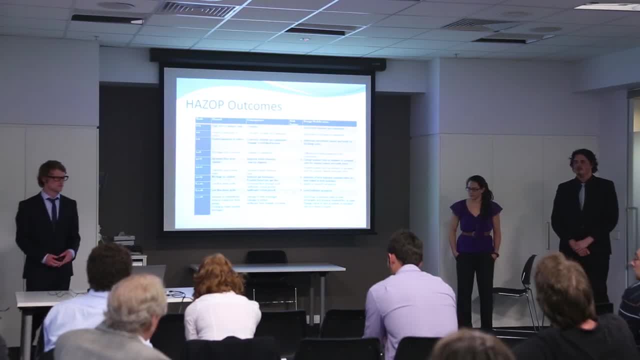 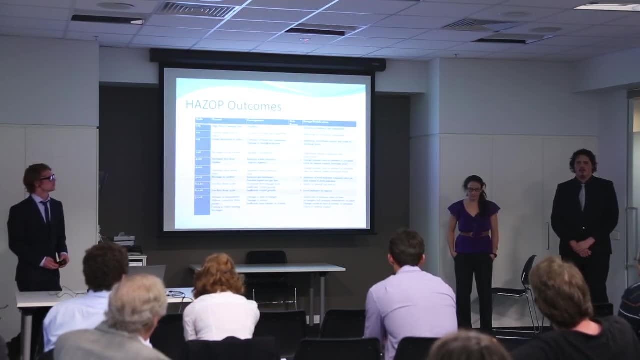 Yeah, that is inclusive of all that sort of stuff. Yeah, maybe I'll have to have a look at the spreadsheet. I need to be able to show that it comes down to like $8,000 an hour. It's not highly creative. 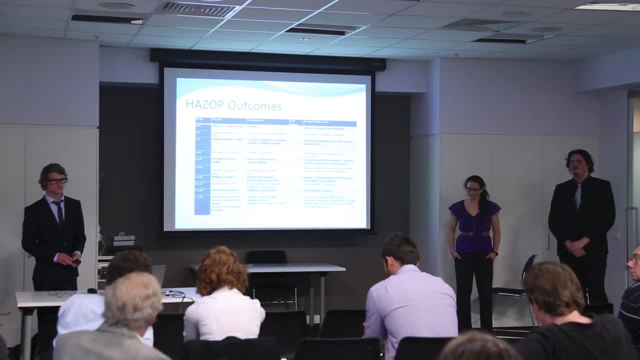 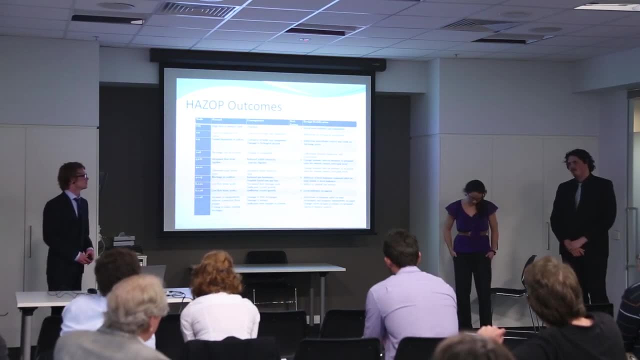 Any more questions? How much CO2 did you produce from your gas? That's a good question. I haven't actually covered it in this report, as you've seen, But we have calculated it. Yeah, that's right. I guess a question from that would be: you could also look at the greenhouse gas impact of the system. 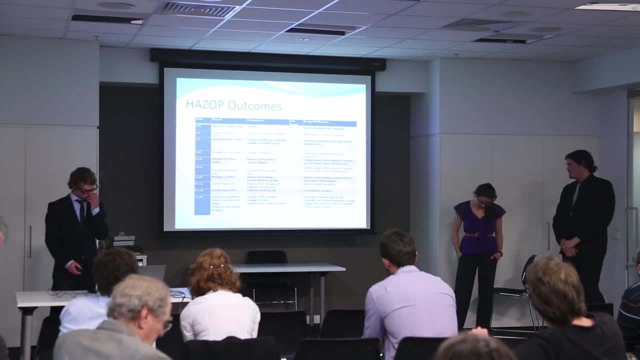 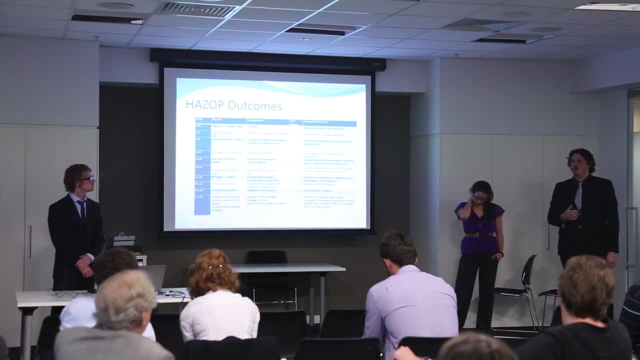 We have looked into that Currently. if you want to compare the overarching company that would eventually control this, compare that to Hunter Water. Hunter Water is just on the lower limit for their greenhouse gas tax, So they're actually almost there, And Queensland Urban Utilities, who covers this area for wastewater treatment, is much smaller.